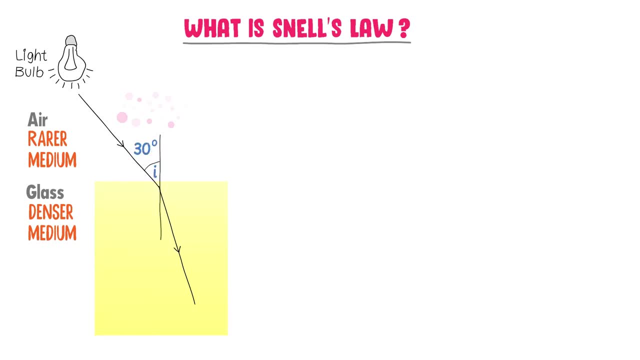 Let the angle of incidence ��otta be equal to 30° in the air and the angle of refraction r is equal to 19.5° in the glass. Now consider second case. An incident ray is traveling from the air into the glass. Let the angle of incidence �idal seb Xc in the air is equal to 19.5° in the glass. Let the angle of incidence ·Cavetta be equal to the angle of incidence ·I is drawn on the glass surface. Let the angle of incidence ·R is drawn on the glass surface. 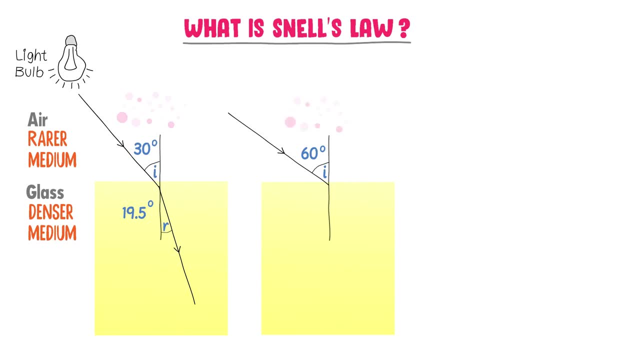 equal to 60° in the air and angle of refraction r is equal to 35.5° in the glass. Consider one last case, in which incident ray is travelling from the air into the water. Let the incident ray I is equal to 50° and angle of refraction r is equal to 36°. 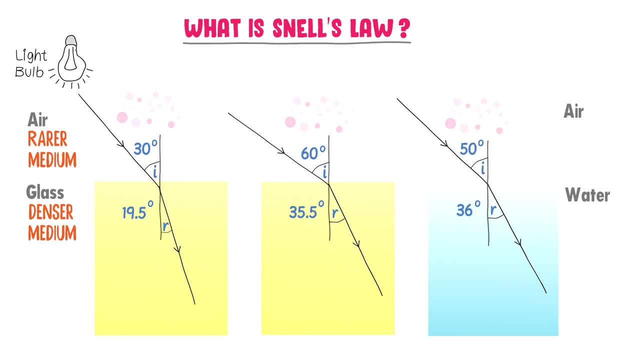 Now, what is Snell's law Here? Snell's law states that the ratio of the sign of the angle of incidence to the sign of angle of refraction remains constant until medium is the same. Let me repeat it: The ratio of the sign of the angle of incidence to the sign of angle. 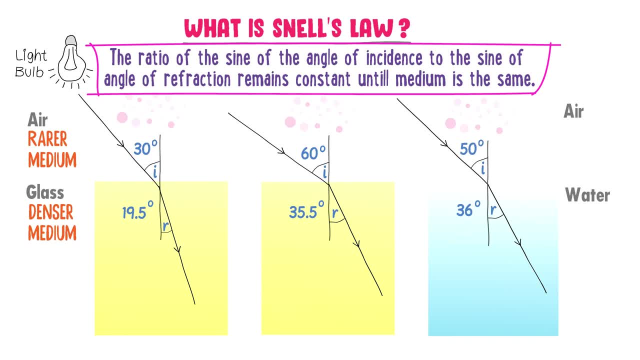 of refraction remains constant until medium is the same. For example, in the first case the incident angle is 30° and refracted angle is 19.5°. So sine 30 upon sine 19.5° is equal to 13.5°. 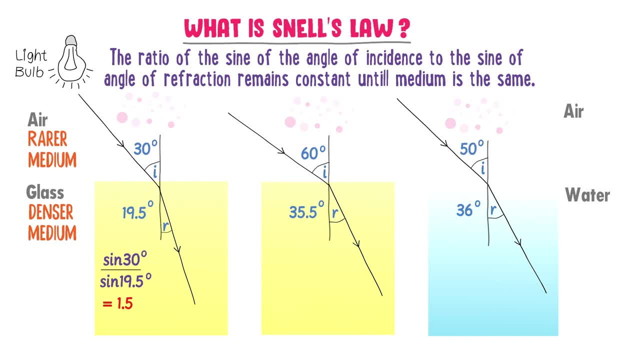 Similarly, in the second case the incident angle is 60° and refracted angle is 35.5°. So sine 60 upon sine 35.5° is equal to 1.5.. While in the third case the incident angle is equal to 50° and the air and the angle 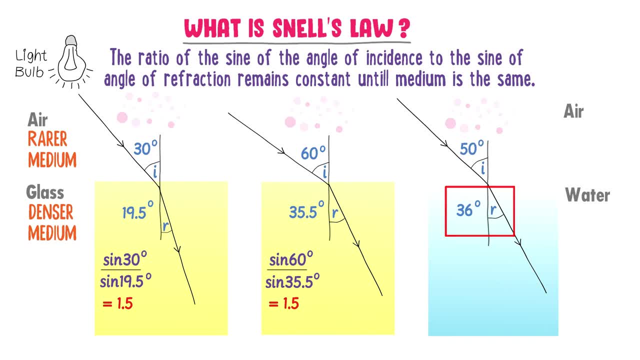 of refraction r is equal to 36° and the water So sine 50 upon sine 30.5° is equal to 30.5°. Similarly, in the second case, the incident angle is 60° and the refracted angle is 35.5°. 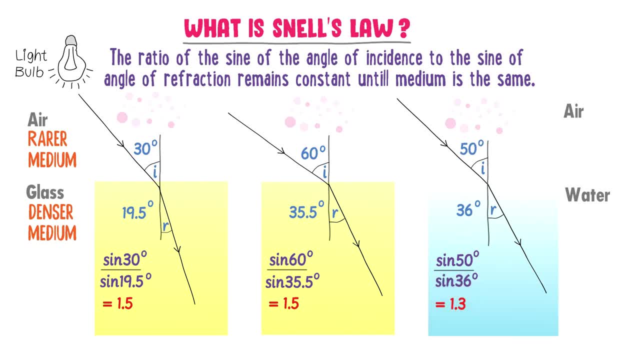 36 degree is equal to 1.3.. Thus Snell's law accurately states that the ratio of the sine of the angle of incidence to the sine of the angle of refraction is constant until the medium remains same. In the first case the ratio is 1.5.. In the second case, the 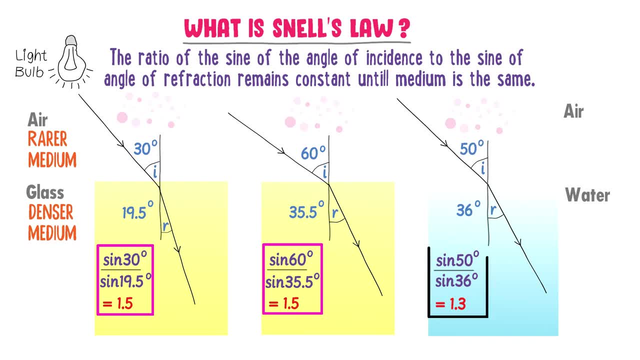 ratio is again 1.5.. But in the third case the ratio is not the same, It is 1.3.. This is because in the first and second cases light is in the same medium. I mean in both the cases light is entering into the glass. So the sine ratio of incident angle and refracted 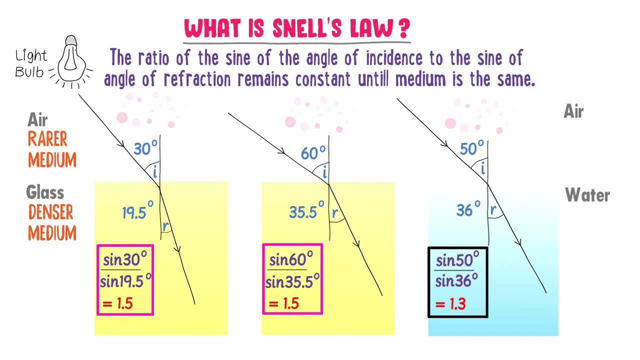 angle remains constant, While in the third case the light is entering into a different medium, like in the water. Thus the sine ratio of incident angle and refracted angle remains constant until the medium is same. Remember that, And this constant value, 1.5, is called refractive index. A refractive index indicates the speed. 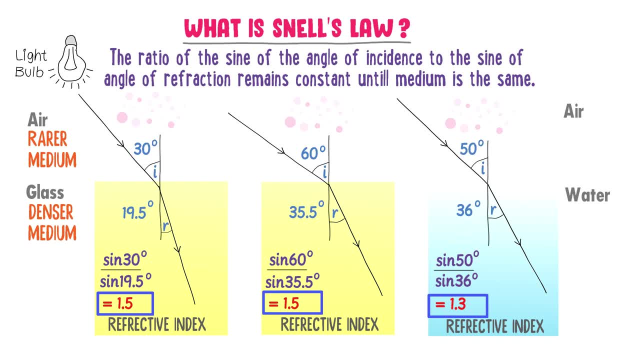 of light. in different media It is denoted by n. When the refractive index is greater, then the speed of light is slower. We will learn more about refractive index in upcoming videos. Therefore, note it down that The ratio of the sine of the angle of incidence to the sine of angle of refraction is constant. 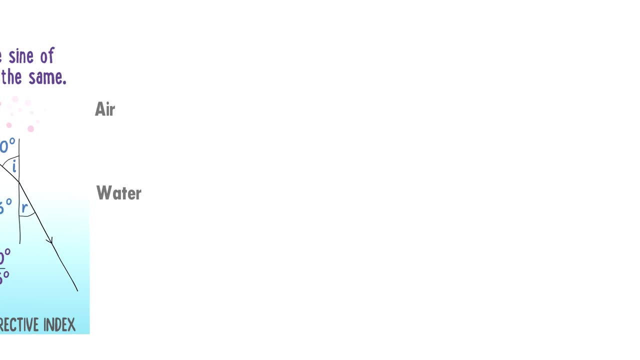 until the medium is same. The ratio of light to the angle of refraction is constant until the medium is same. Let me teach you the full concept of Snell's law, which we study in our school or college. Let's consider that incident: light ray is coming from the air and hitting the surface. 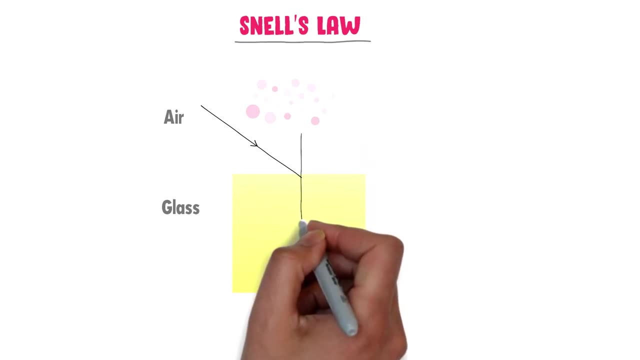 of a glass, We know that the incident ray will always bend towards the normal. in this case, Let the incident angle. I is equal to 30° and the angle of refraction R is equal to 19.5°. Now listen carefully. Air is one medium and glass is one medium, So let's. 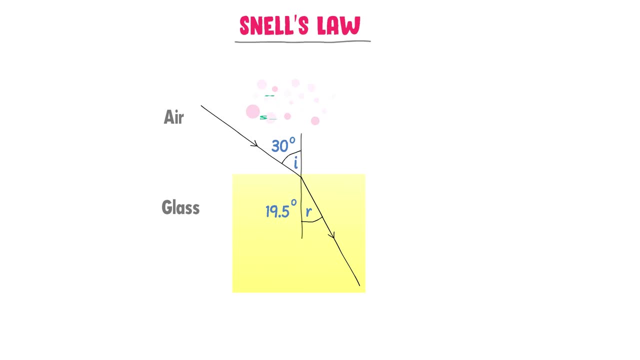 see that, without going any further, We know that incident light ray is coming from the air and hitting the surface of a glass is constant until the medium is level in angle of refraction. glass is another medium. The speed of light is high in the air and the speed of light 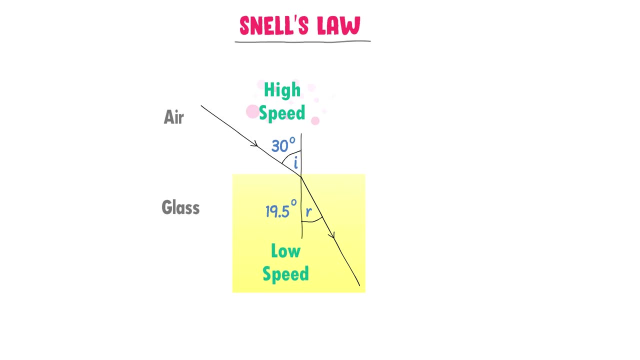 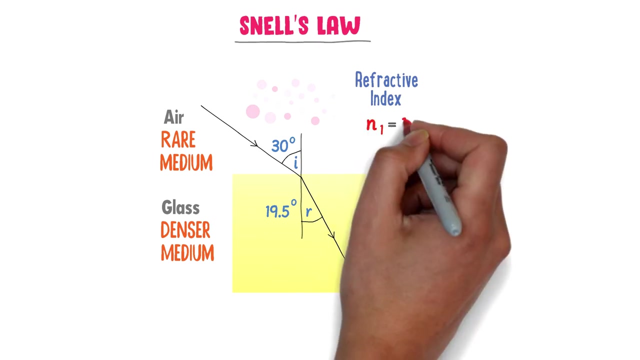 is slow. in the glass, Due to this change in speed, light is refracted. So we say that optically air is rarer medium and optically glass is denser medium. Now, as a standard we say that the refractive index of the air is n1 is equal to 1.. What about the refractive? 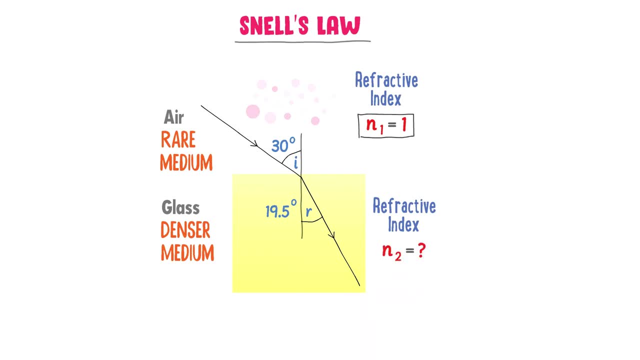 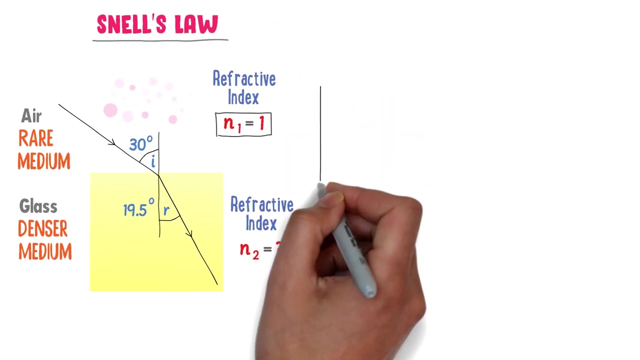 index and 2 of the glass. Well, we can guess that the refractive index of the glass will be greater than 1, because glass is more optically denser medium. But how we can find the refractive index of the glass? Here we use Niel's law. It states that sine ratio of incident angle. 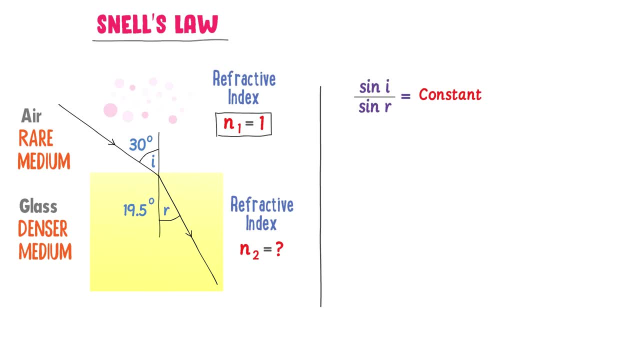 and refracted angle remains constant or it is equal to refractive index. Now, instead of this constant, I will put the refractive index of air and glass in the Snell's law. So sin i upon sin r is equal to write the opposite refractive. 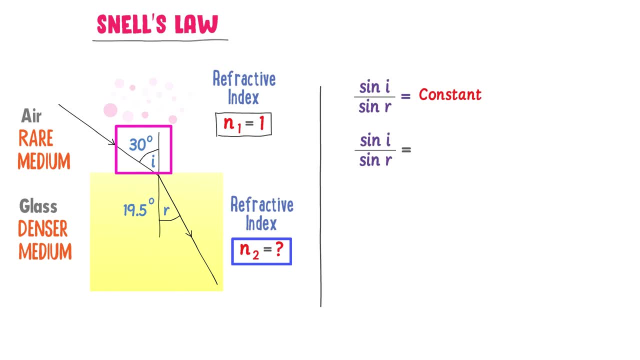 index to incident angle i. It is in the air, so I will write the refractive index of glass, n2 in front of it. To sin r, I will write the opposite refractive index- I mean refractive index of the air- n1- in front of it. This is one method of writing Snell's law. Let me 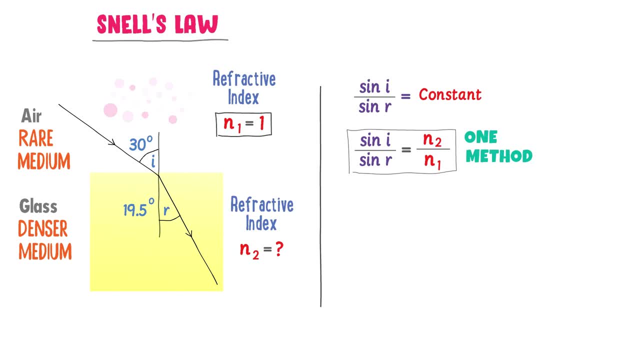 also teach you my personal and fast method of writing Snell's law. I divide this diagram into two equal parts. This is upper part and this is lower part. Firstly, I write upper part as n1- n2- sin i at one side of the equality and then I write lower part, n2- n2- sin r at. 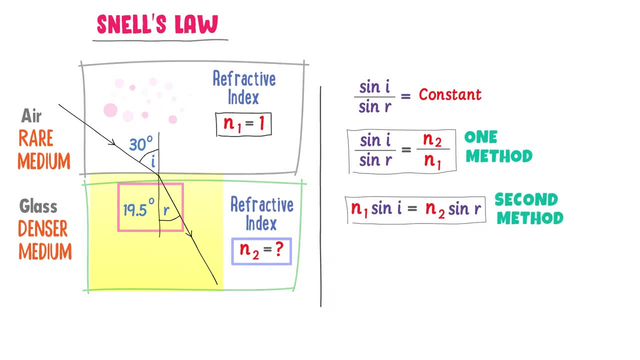 another side of the equality. So this is the second method of writing Snell's law. Now what about the refractive index of the glass? Well, plug in all the values in the Snell's law. After calculation I get: n2 is equal. 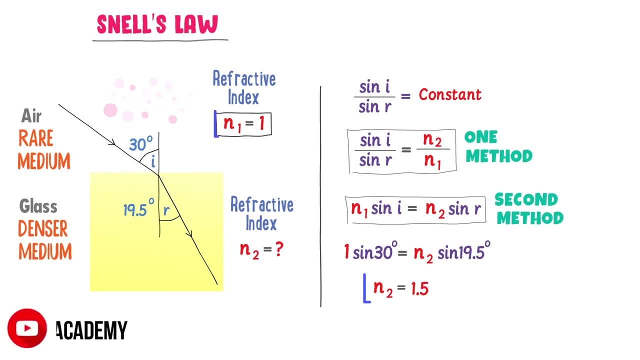 to 1.5.. As I told you, that refractive index of the glass would be greater than the refractive index of the air, So it is 1.5. The speed of light is high in the air because its refractive index n is equal to 1., While the speed of light is low in the glass because its refractive 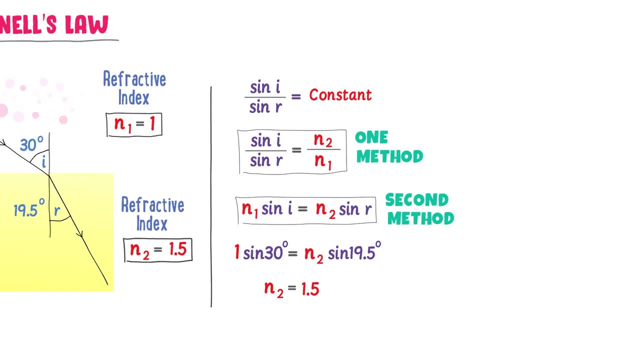 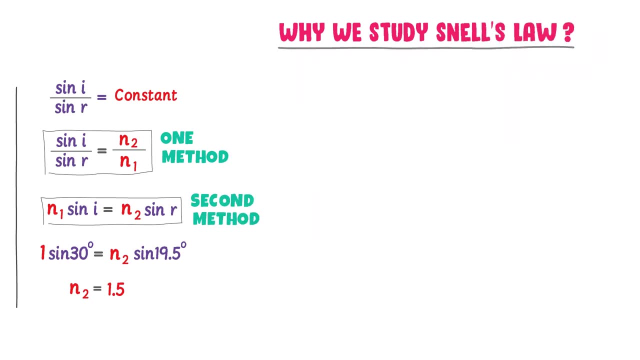 index n is equal to 1.. So it is 1.5.. Now let me ask you why we study Snell's law, or why we need Snell's law. Well, the answer is very simple. It is due to three reasons. Firstly, we need Snell's law to find the angle.